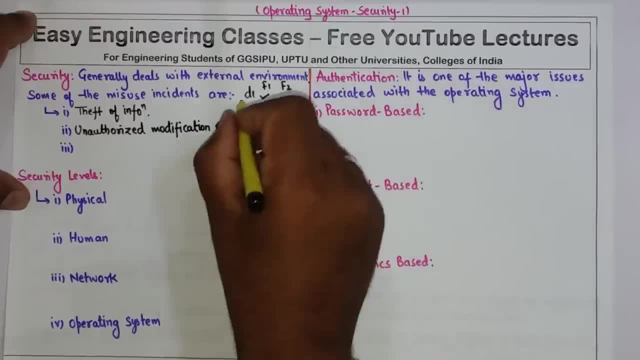 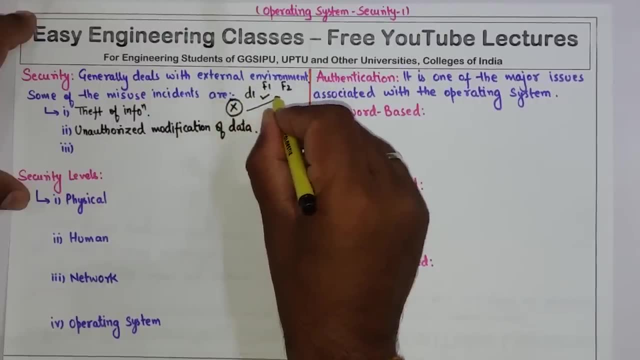 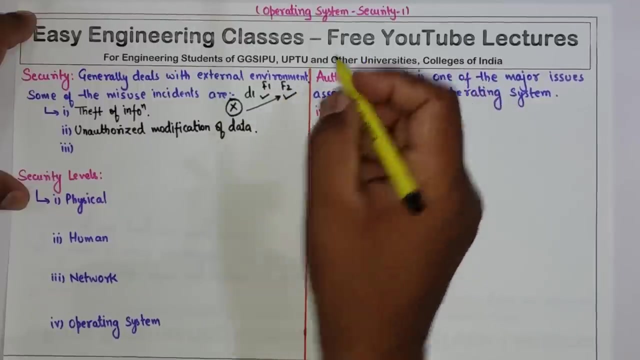 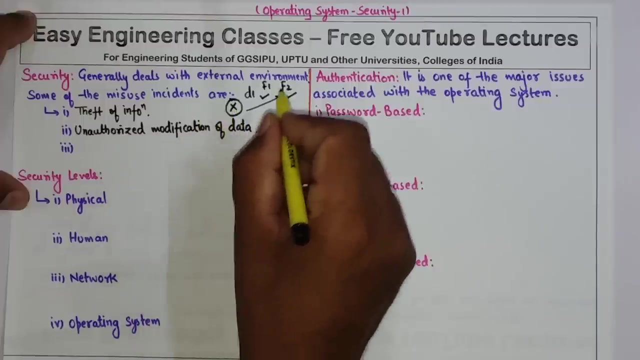 executing in domain D1 can access files F1.. Now there is a attacker X external to the system and that attacker intentionally changes the domain access matrix and gives the permission of this also. So by this, This X is unauthorized. This X, which is unauthorized to perform any modification to this access matrix, is modifying. 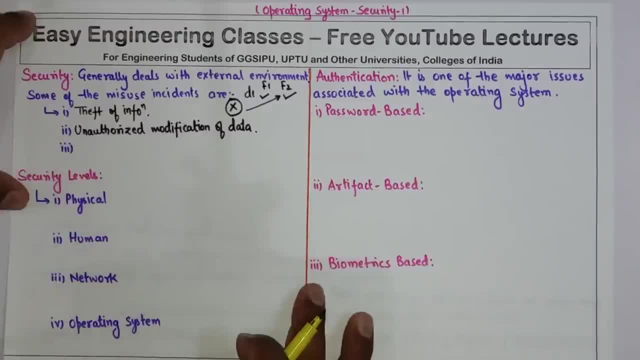 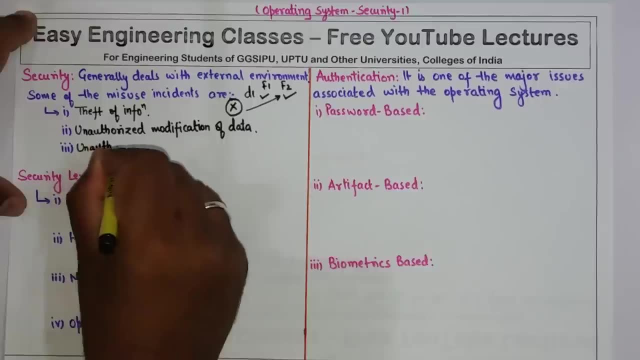 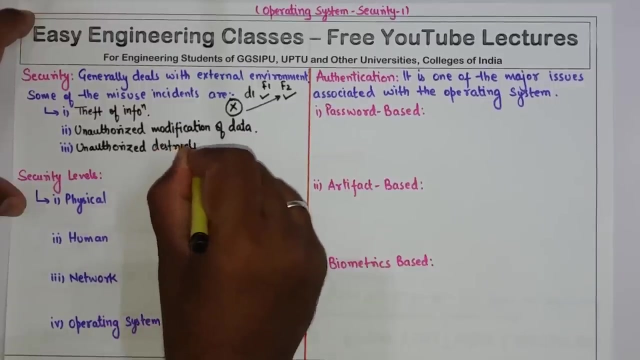 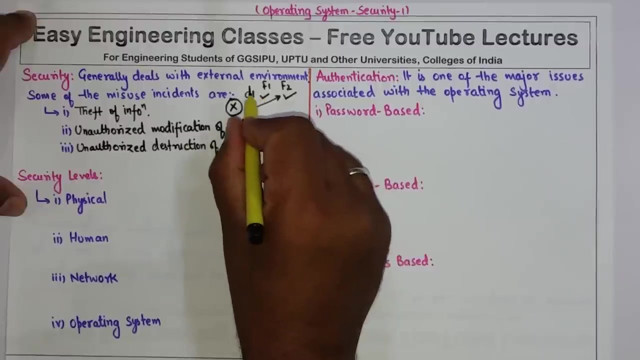 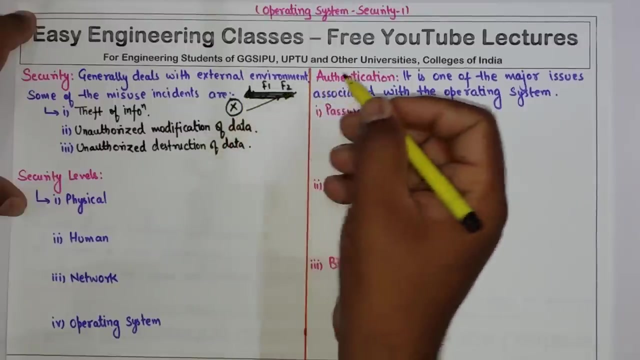 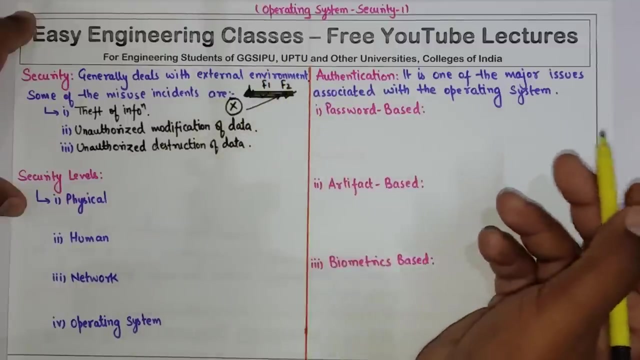 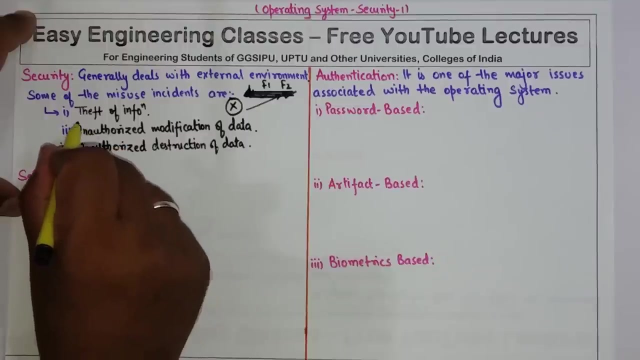 it and that is a external threat to the operating system. Now, third can be unauthorized, unauthorized destruction of data. So, similarly, if this DA Magical can also be used for the tossing of esteemed data, so forth, Now what is the consequence? The consequence of this, if 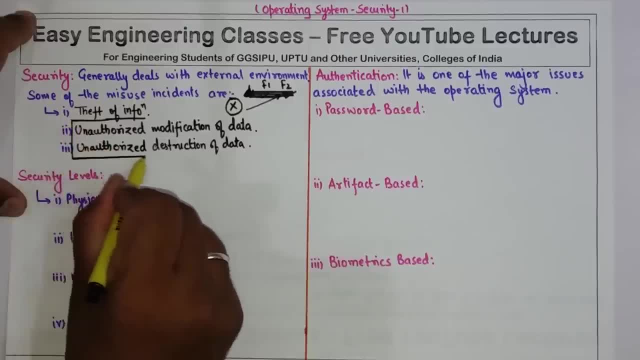 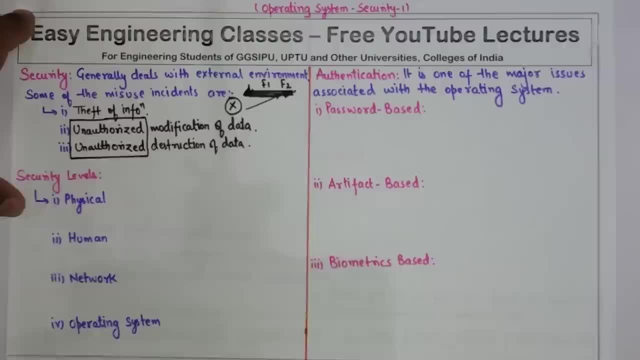 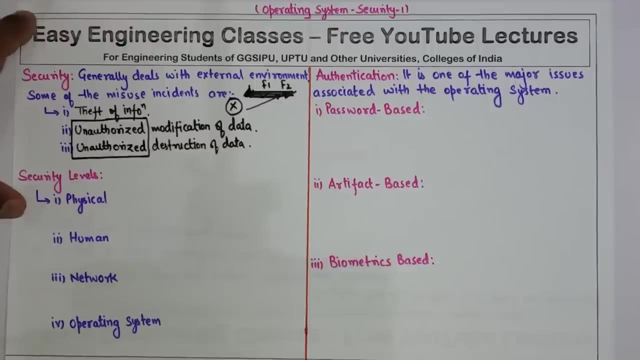 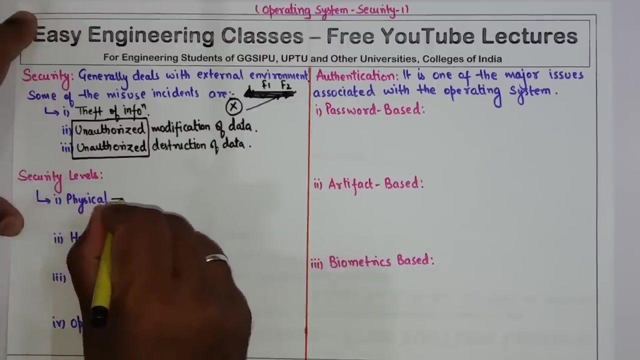 Proigkeit futures an audiences records are anything perform modification and destruction of data. but if the user is unauthorized then that comes under the external threat of the security breach. now there are different security levels. first is the physical level. now the site containing the computer system must be physically stored. 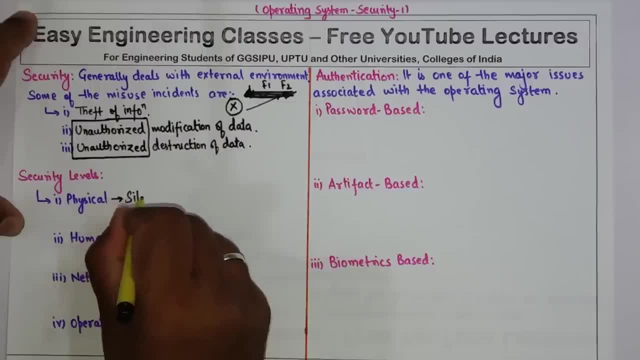 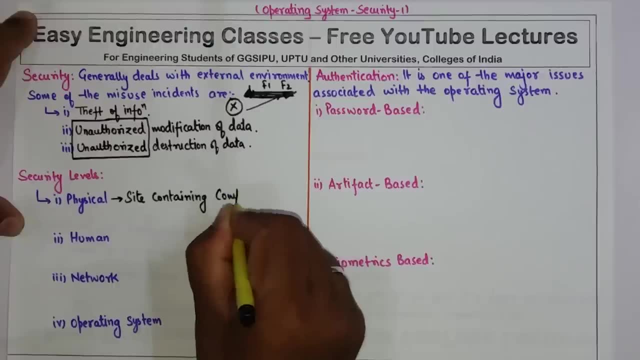 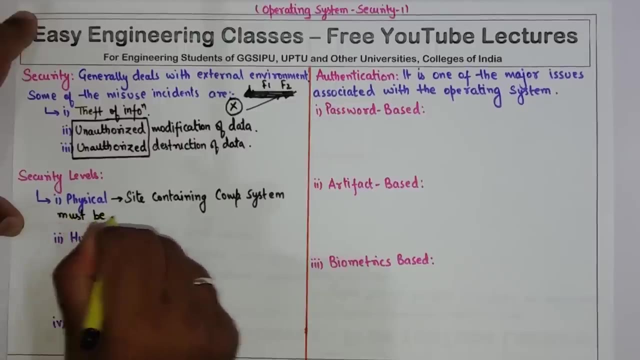 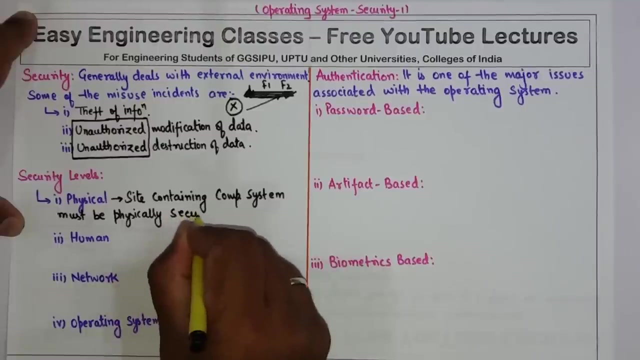 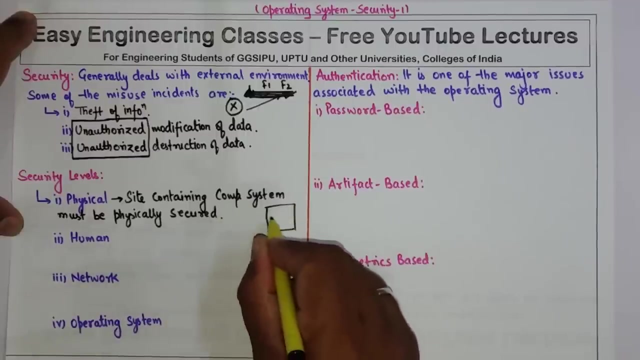 so site containing the computer systems must be physically secured. now in this you can take an example of a bank. so what happens in bank is that there are security guards outside the computer system and when there is a security guard, that guards inside the bank and these security guards prevent any kind of malicious user from entering into. 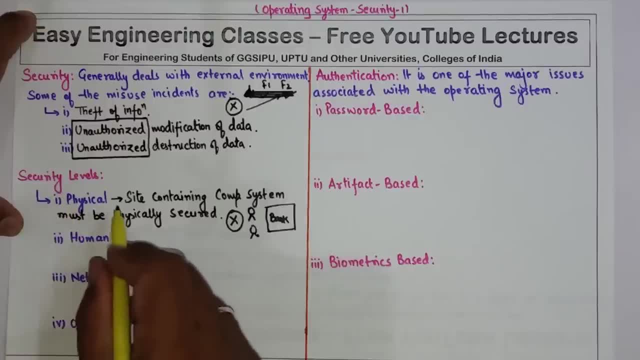 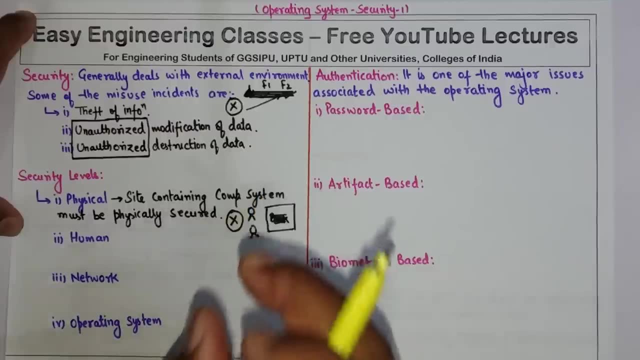 the bank. Now, same goes with this operating system security level. So if we have a computer system here at a site, at a place, then there should be the physically security measures should be implemented so that any malicious user is stopped from entering in this building. 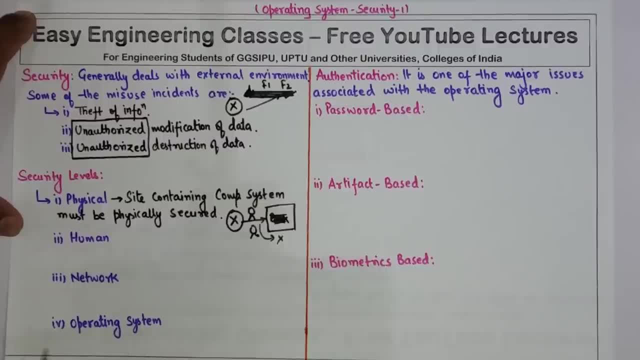 So this is the physical security level. Now the next is human. Now even the permitted user should be carefully screened so that the chance of authorizing a user who may give access to the intruder is reduced. So the human. we can say that we should have certain kind of authorizing mechanism implemented. 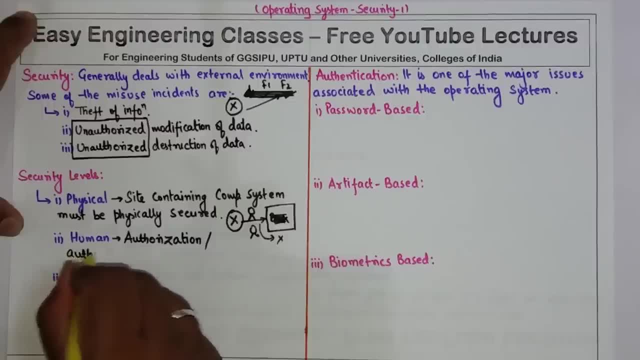 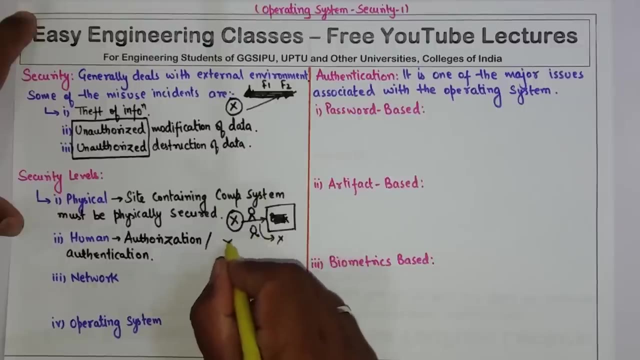 Authorization Or authentication mechanism should be implemented so that a normal user can be distinguished from the intruder. So you can take an example of this also. suppose if a user y enters into the bank and tries to access the mainframe of the software installed in this bank, then that should be stopped. 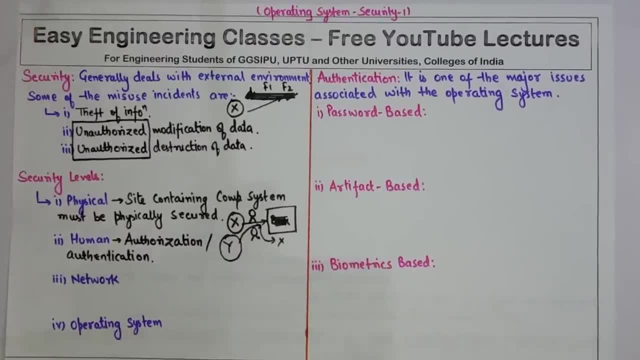 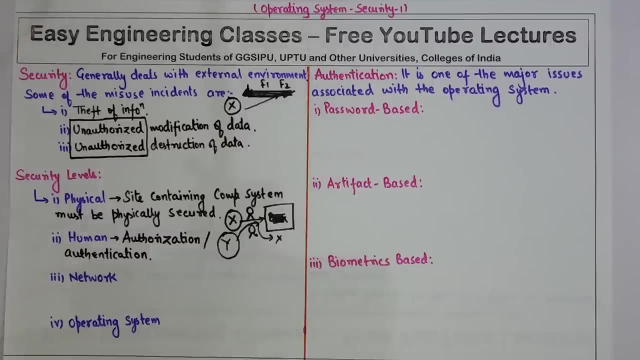 But third level of security is network level. Now in modern days there are the data normally travels through the internet. So there are certain lease lines, shared lines like internet, or in India there are dial up lines also. So the interruption of these communications should be remote denial of service attack. 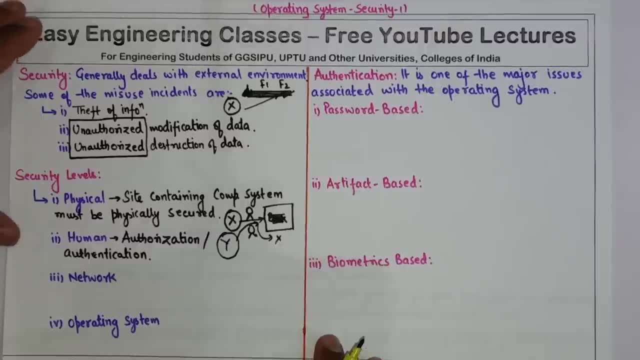 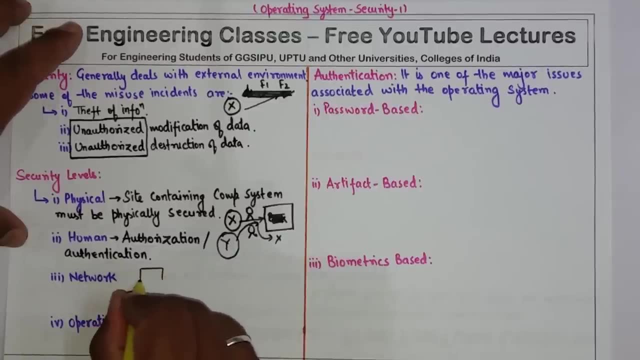 or the interruption of the internet. So in this case the interruption of these communications should be remote denial of service, attack and others. so this should be secured. so, for example, if i say there is a data traveling from this site to this site and in between we have this network, so this data, this message. 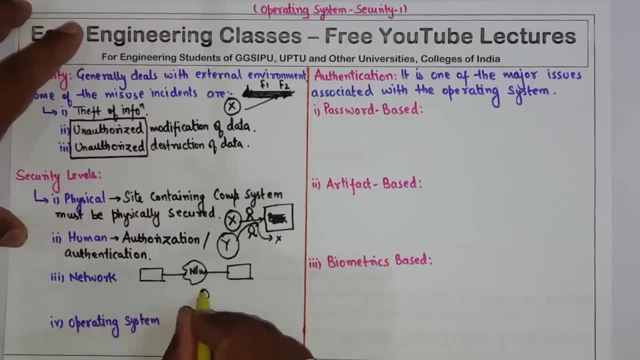 should be properly secured so that a intruder or the malicious user sitting in between these two sites cannot access to this data. so in this the concept of encryption comes into play, which we are going to discuss later in this tutorial series. the last level of security is the operating system. now the system must be protected itself from accidental or purposeful 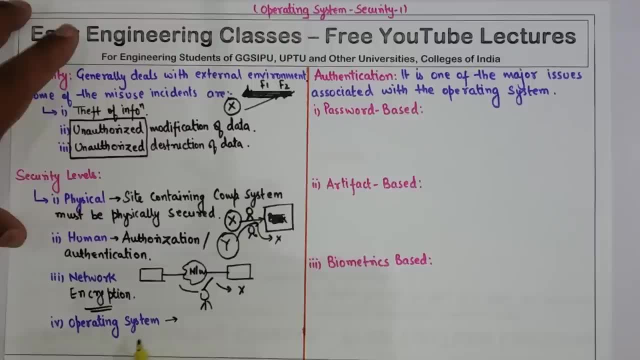 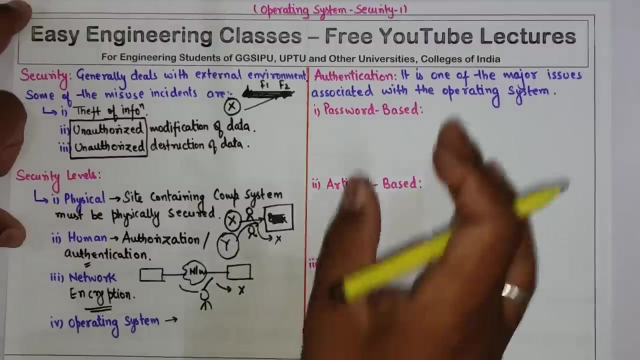 security breaches. so we should have certain security level installed in an operating system so that it should be protected from itself accidentally performing some security breach operations. so this is different security levels of operating system. now, as we I have already told you that the authentication plays a very important role in security. there are three different kinds. 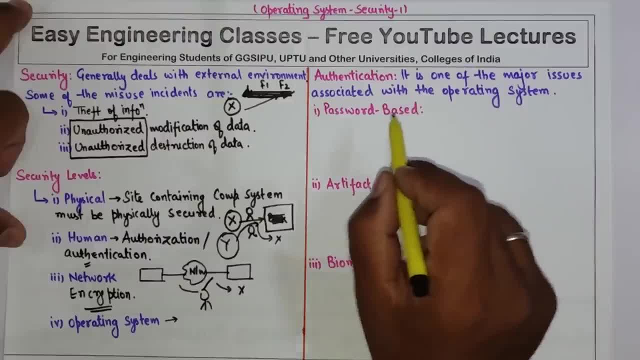 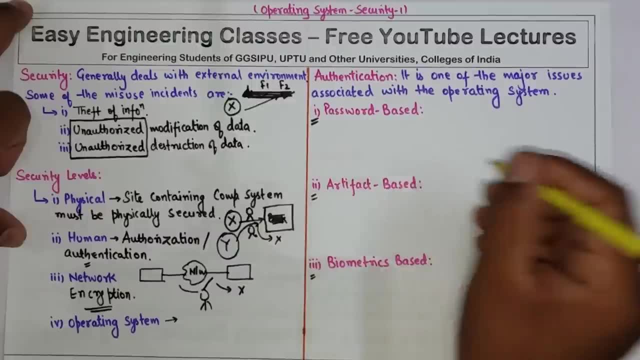 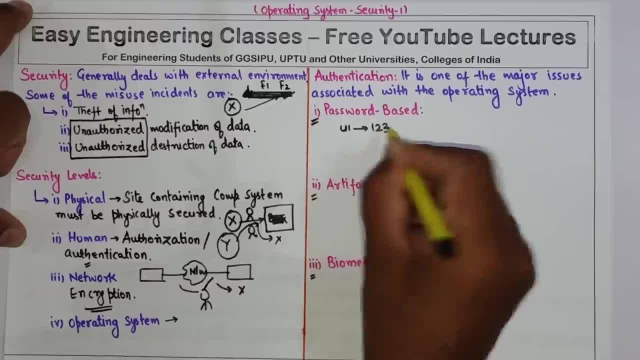 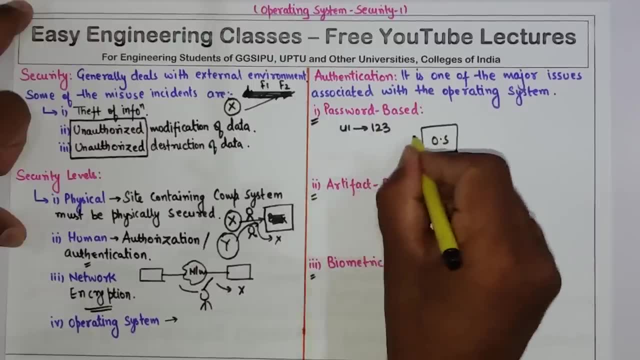 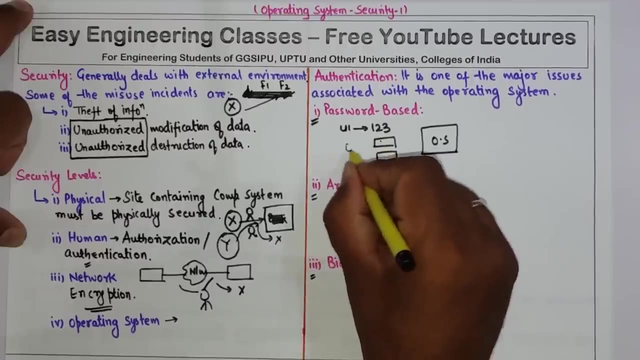 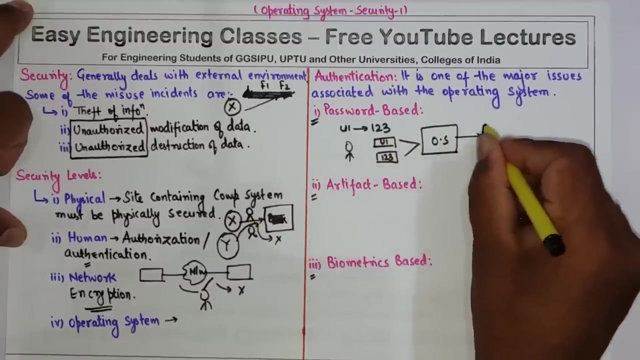 u1 and the password of user u1 is u123. now, whenever this user wants to enter into the operating system, that operating system asks for the username and password. so suppose this user enters u1 and 123, so then this OS checks this user ID and password in the database stored inside the operating system. 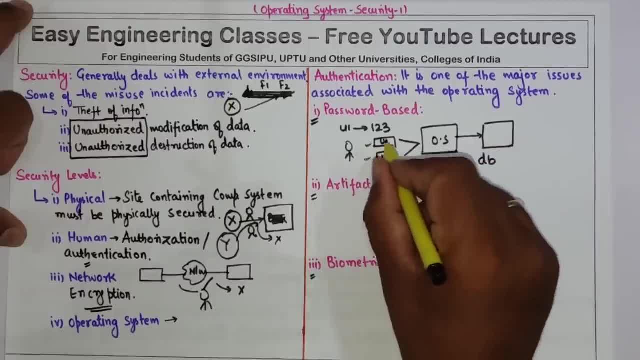 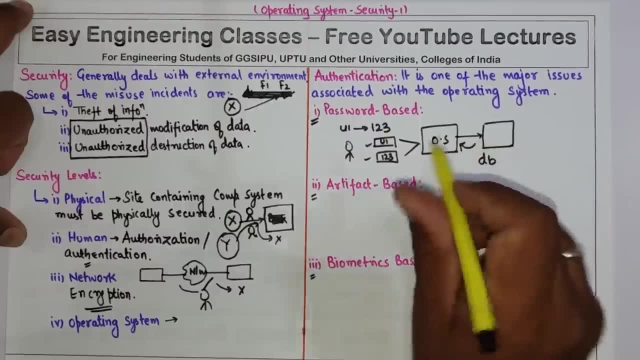 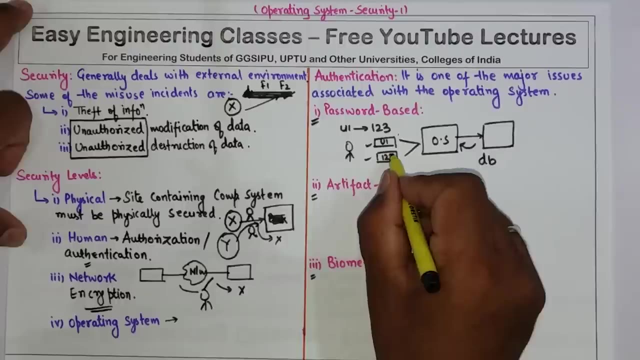 files and if the match is made that for user u1 the password is 123, then a success is written from the database OS and this OS will grant access to this user. now if the user u1 enters one, two, then this will return false and this user 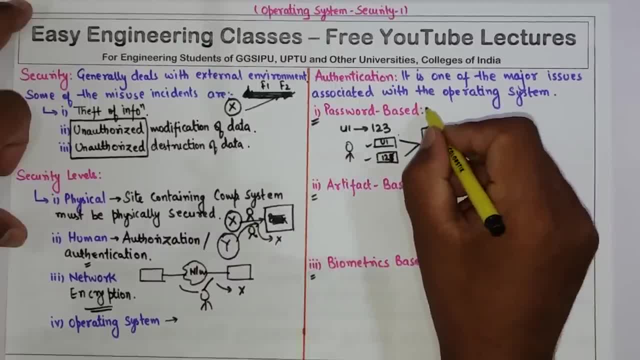 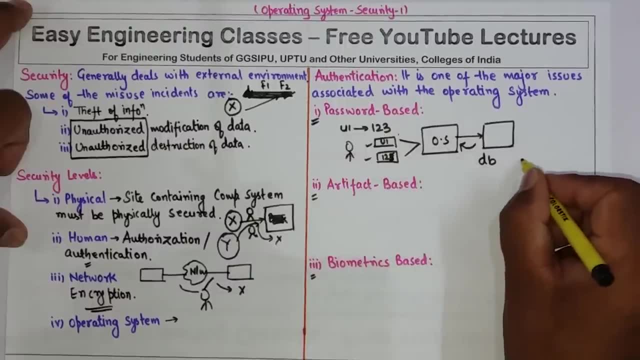 is not allowed to enter into the OS. the problem with the password based mechanism is that normally the passwords are stored in plain text files. so if a attacker or the hacker somehow gets access to this database containing all the username and passwords, then then attacker can gain access to. 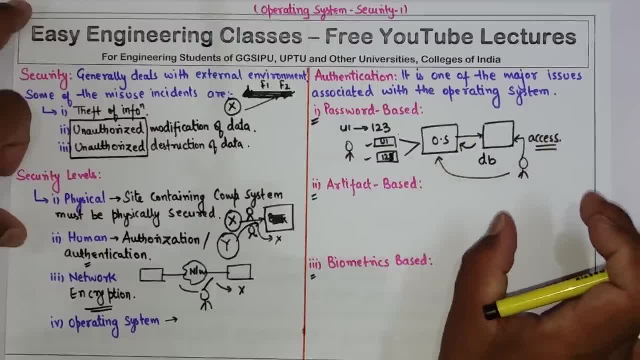 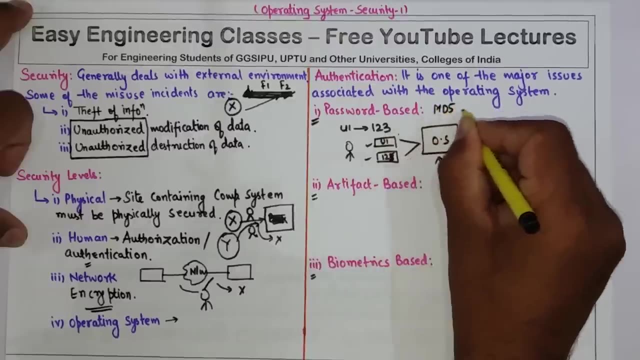 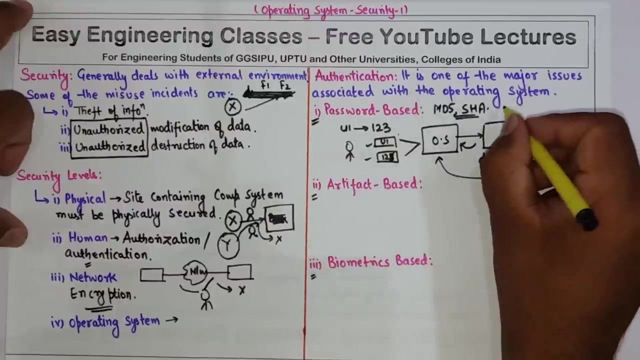 this OS imposing as the legitimate user. so this is one of the main problems of this password based mechanism. there are certain algorithms implemented for the security of this password base. also, like we use MD5, SHA, which are hash, so instead of storing the password as plain text, the hash. 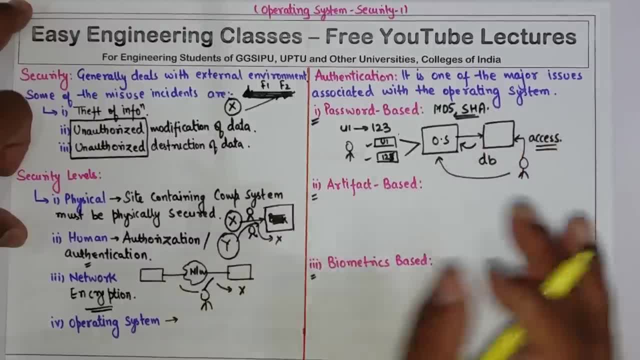 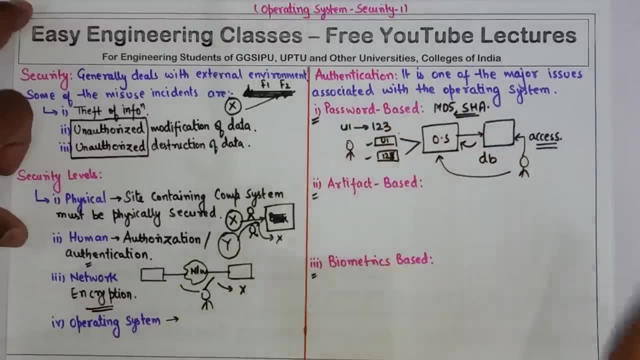 value of that password is stored in the database. so that is a security topic which I have already covered in the computer network security. so if you want to study in detail you can refer that video. but as per the operating system part is concerned, this is enough, that password. 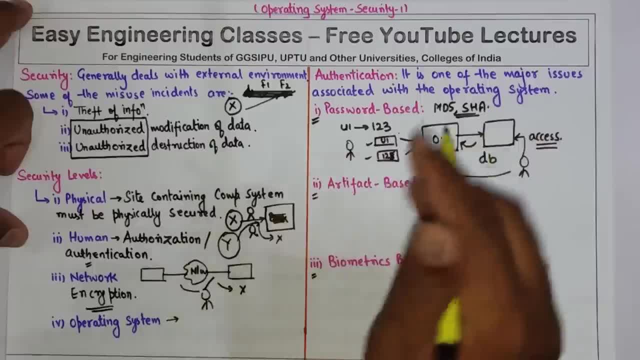 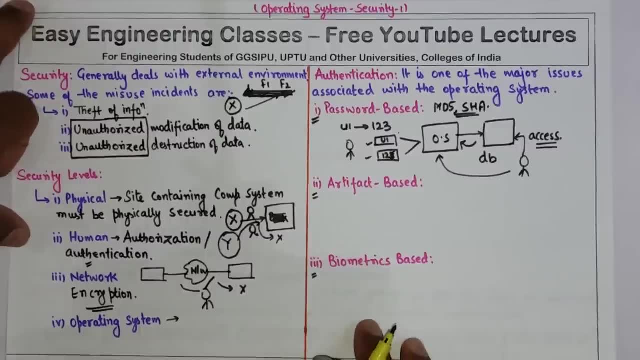 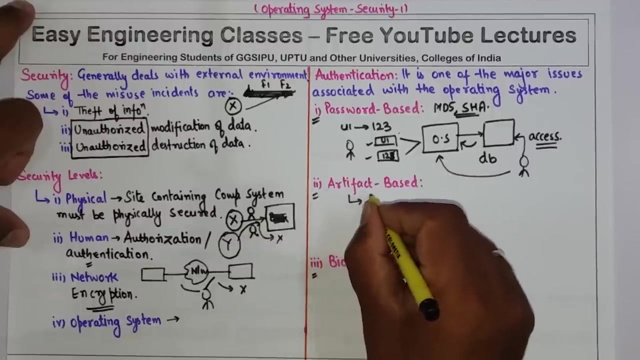 based mechanism works like this and, to make it more secure, we can use hessian techniques like mt5 and sh shm. now, second type of authentication mechanism can be artifact based. now, artifact based authentication mechanisms includes machine readable strips or magnetic strips, and this can be smart cards, debit 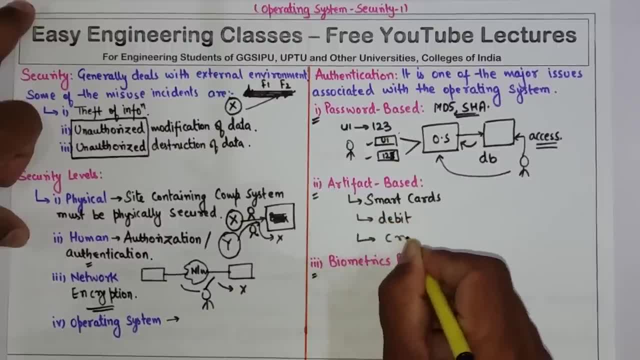 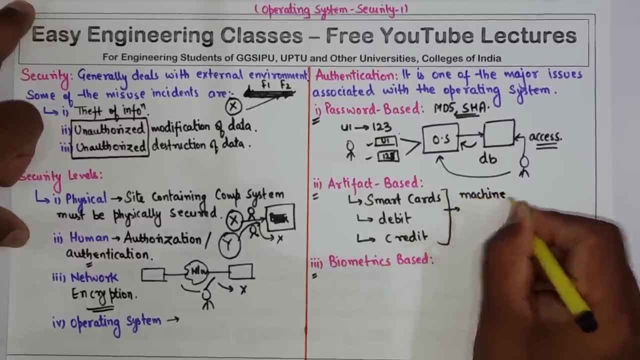 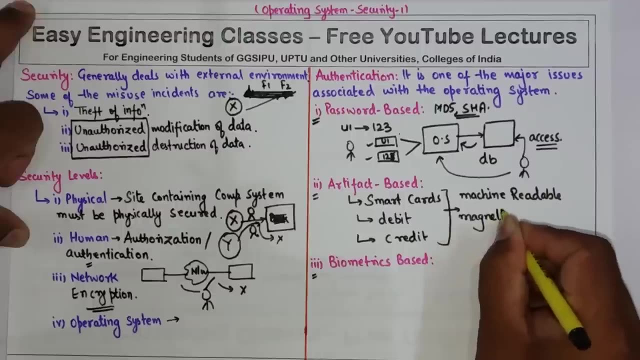 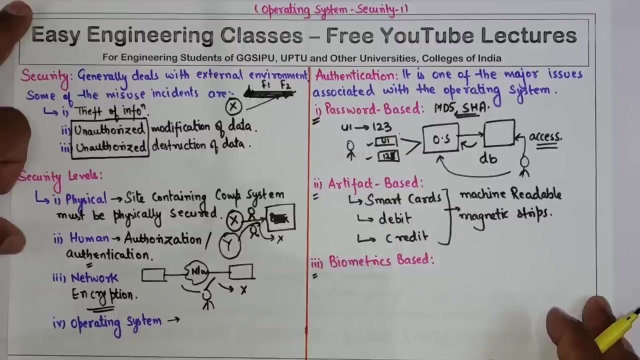 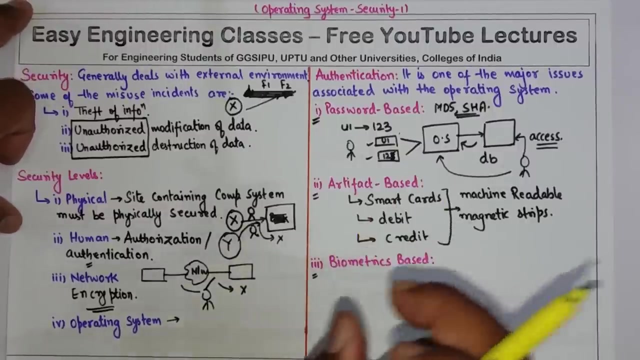 cards, credit cards, and all these cards contains machine readable magnetic strips. these are the artifact based authentication mechanisms. now card readers are installed in the company and user or the employee is required to supply the artifact, which can be smart card or any other card, for the authentication purpose. the last is the biometric base. it is considered as one. 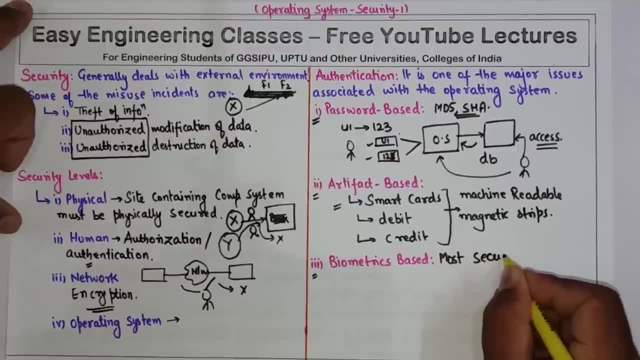 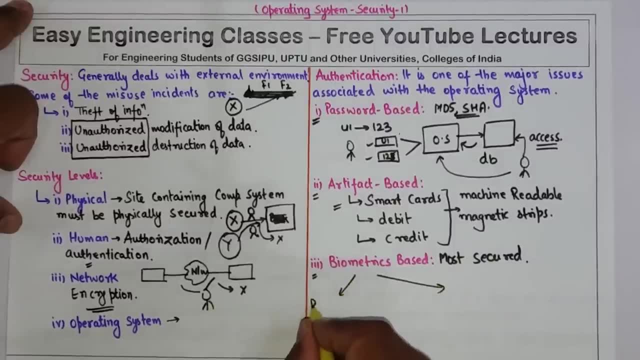 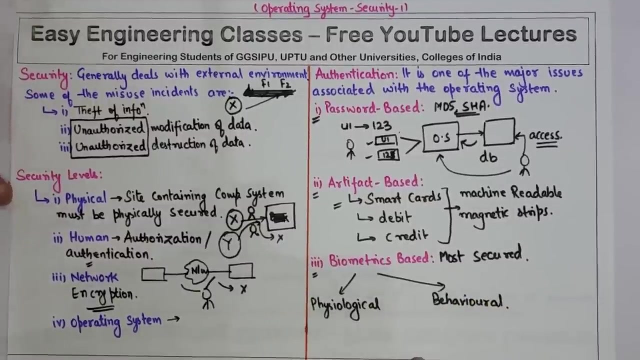 of the most secure authentication mechanisms in the market. these are the different authentication mechanisms. it has two characteristics: one can be physical and another is behavioral and, depending on these two different kinds of characteristics, there are different biometric authentication mechanisms which are employed for the authentication purpose, not the physiological means. 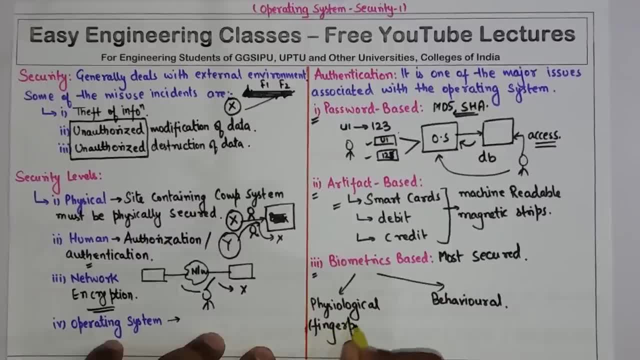 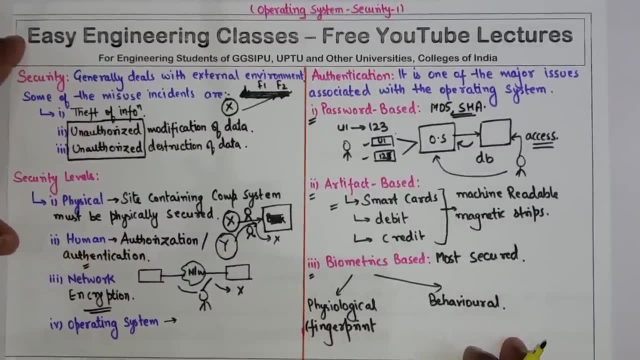 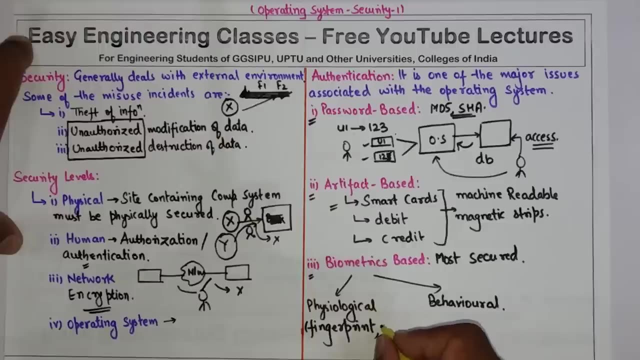 fingerprint. the biometricWellington gets the identification data and these, the most commonly used biometric, is the print of your finger or the thumb in the common cases. other kinds of physiological characteristics can be retina and face. so these are the physiological biometric mechanisms, behavioral means, signature dynamics.